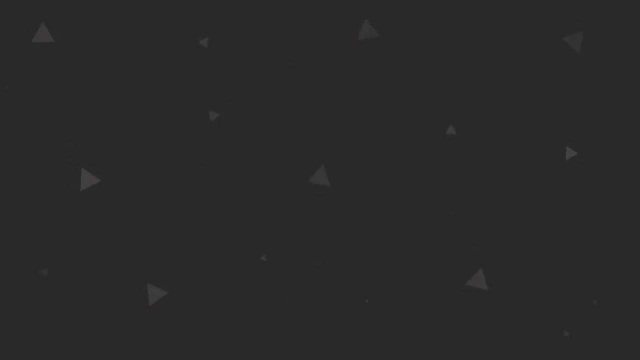 episode with which I think it's going to be much better workflow because, first of all, you're using github, not git that you get with c panel, and we are going to be using github actions Now. this approach is much better because, of course, because with github you get much more options with your. 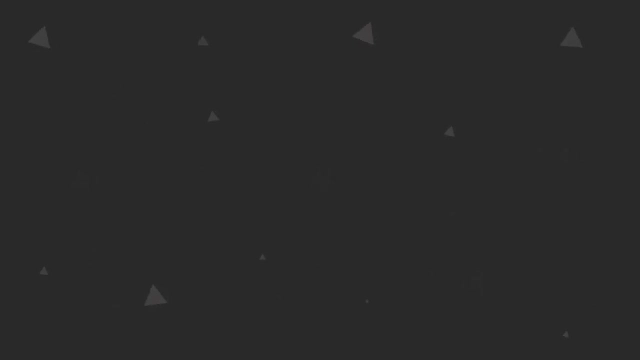 code versioning and also it has github actions and and it's much nicer to use. So in this episode we are going to use github actions and github to deploy our website to the shared hosting. That website is going to have a staging brand branch and the master branch, So the master branch is going to go to our production. 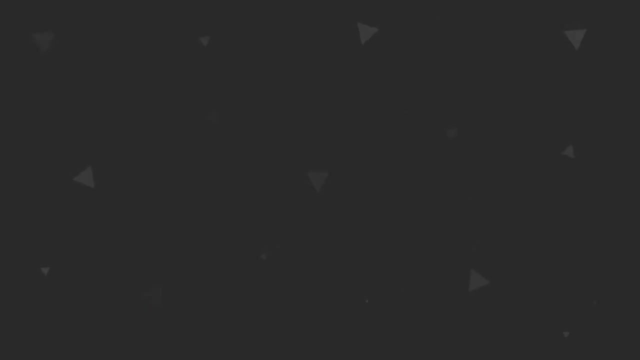 and the staging branch is going to go to our staging server where our clients can see the changes that we made and if they approve them, then we can push those changes to the production or to or to the live website. So that is what we are going to be doing in this episode. 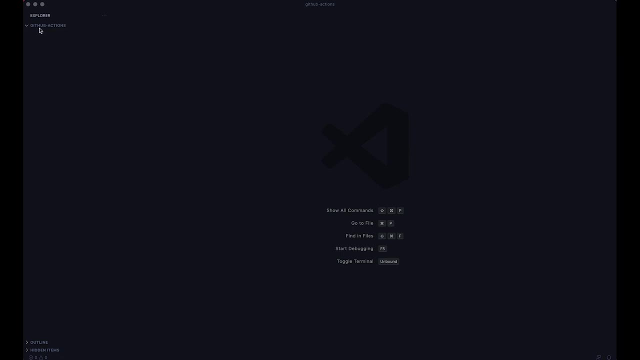 So, first of all, let's create our project. I'm going to call it my project: github actions. I'm going to create a new file in it and I'm just going to call it indexhtml, and in it I'm just going to put some 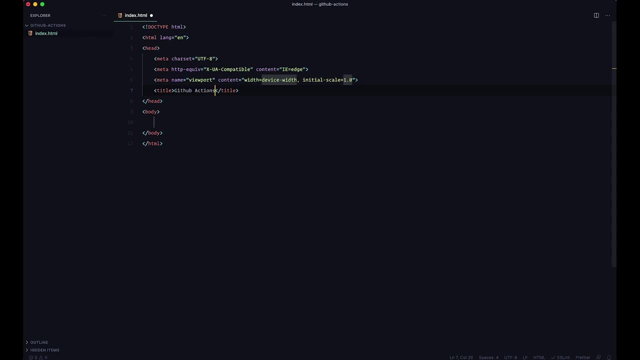 boilerplate code and change the title to github actions, and we are just going to add an h1 tag and call this. this is our production, because this is going to be in our master. So this is our production. We're going to save this, and now we are going to create a new folder called. 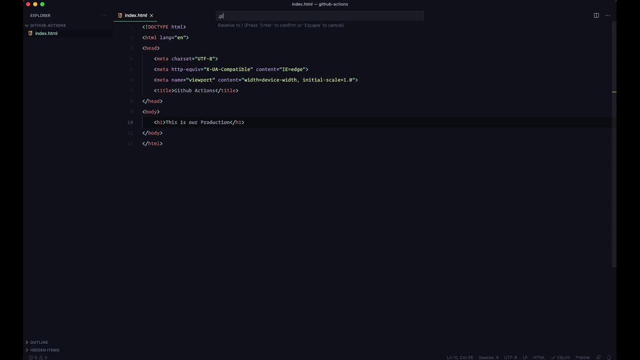 github or dot github, and in it I'm going to create another folder called workflows and in it I'm going to add yml file which is going to be called master dot yml. In here we are going to define our github actions which are going to push. 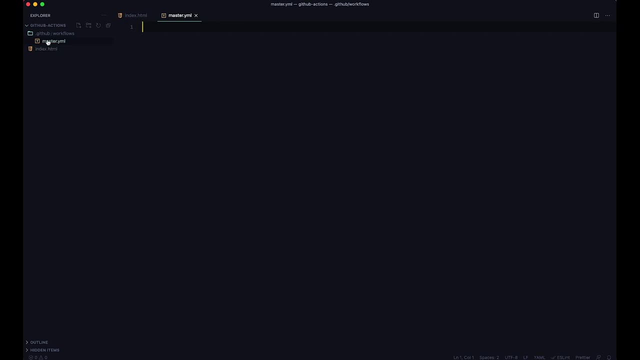 site to our shared hosting. So, as you can see, right here on the left side, you have github workflows and master yml, and also I'm going to call create another file, which is going to be called staging yml. Okay, so now we have these two files. Now what we are going to be using. 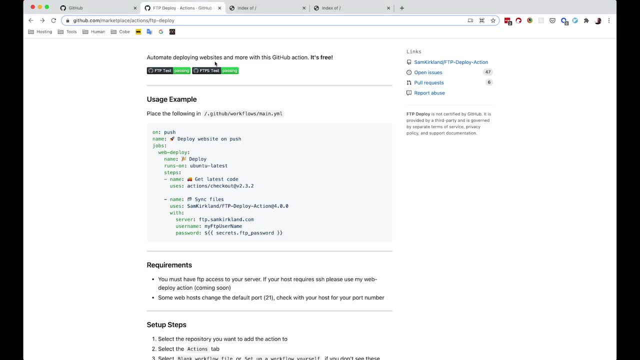 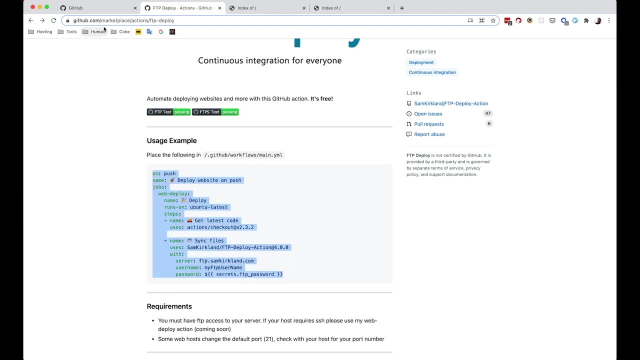 for these github actions is actually this section right here which is called ftp deploy, and I'm just going to copy it. I'm going to copy it to my github account. I'm going to copy it to my github account. Of course, you can find it in marketplace actions: ftp deploy on github. We are going to just copy. 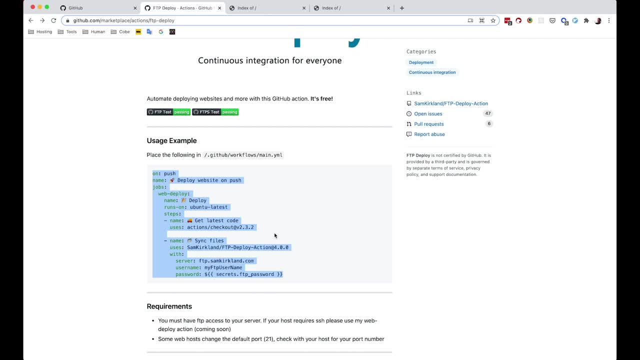 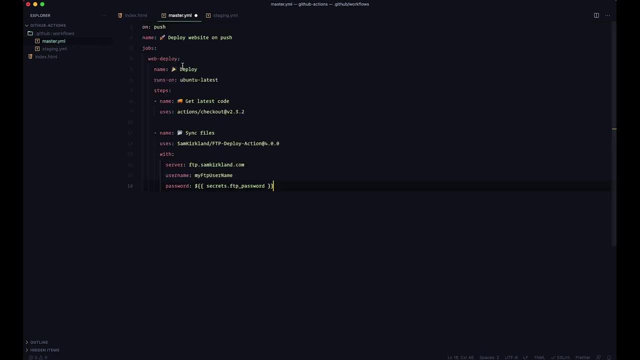 this and then we are going to change some stuff to it. So I'm just going to go to my code editor and in master dot yml, I'm just going to paste this in. and now here it says, on push. So whenever you push something to your github repository, this is going to trigger. Now, we don't want this. 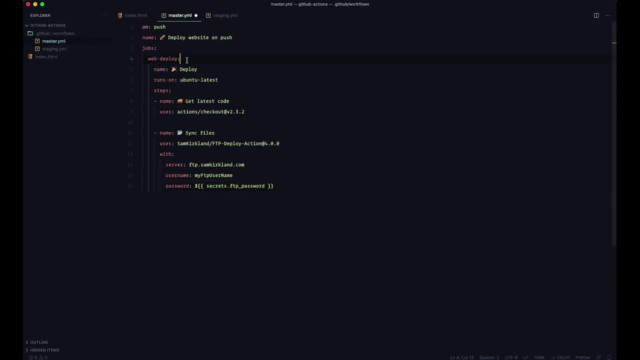 to trigger every time. We only want this to trigger when you push something on the master branch. So instead of doing just on push, we are going to delete push and just leave on. Let me make this bigger, sorry, Okay, so, and now I'm going to say push and I'm going to say branches. 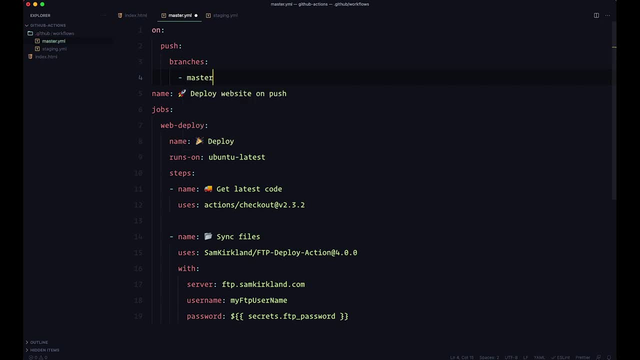 and then I'm just going to say: master, The indentation is very important inside of yml files, so keep an eye on that. So what we are saying right here: when you push something to master, then you deploy my code to my shared hosting. So there are going to be some jobs. web deploy: it's going to get the latest code, sync the files. 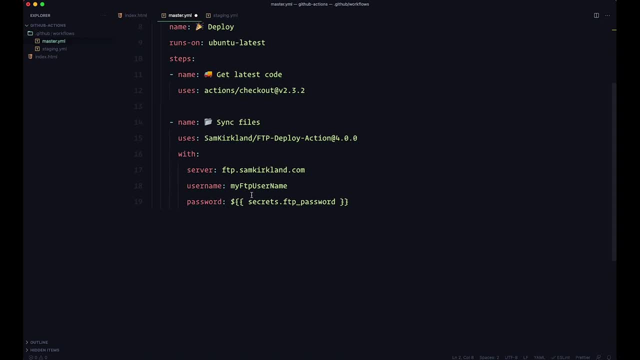 and push them to the server. Now you need to define the server, and in my case that is going to be this: So de3.fm. Of course, for you it's going to be something different. And now, as you can see, for username and passwords we are using secrets, So I'm going to also use a secret for the username. 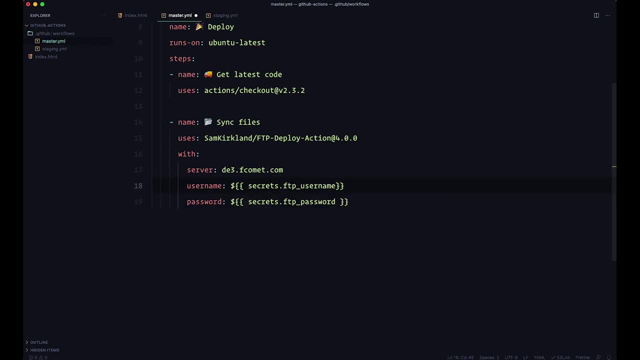 Secrets. So it's going to be secrets- ftp username and secrets- ftp password. And there is one more thing that we need to define. At least I need to define it. You may not need to define it if you are pushing the code inside the root. 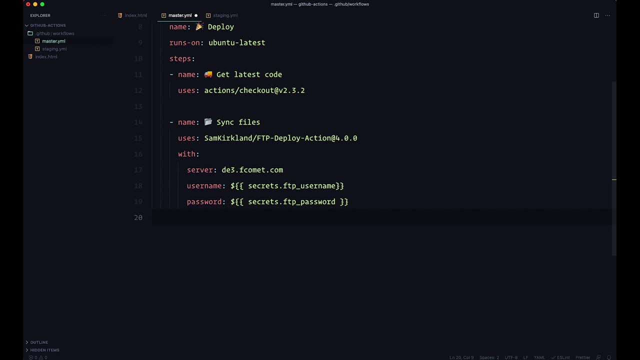 of where you log in with your ftp. But I have to define it right here, and it's going to be called serverdir and it's going to be public html. So it's going to be called public html: productionwatchlearncom. Okay, save this. And so when the master branch is pushed to a repository, this is going to trigger. 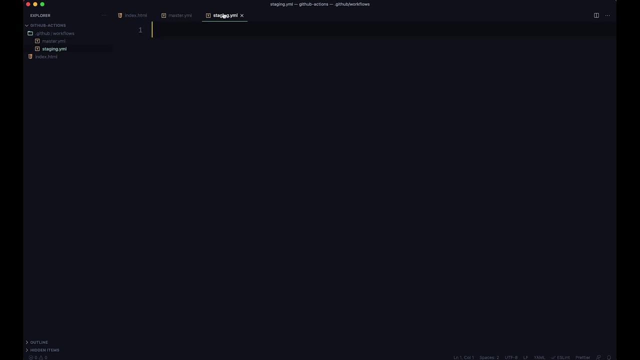 Next, I'm going to copy all of this and just put it on the staging yml and I'm going to call this branch serverdir. This is going to trigger. Next, I'm going to copy all of this and just put it on the staging yml and I'm going to call this branch serverdir. 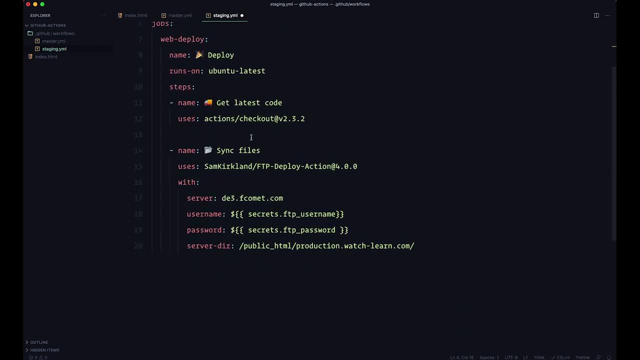 Next, I'm going to copy all of this and just put it on the staging yml and I'm going to call this branch serverdir Okay, and everything else stays pretty much the same, except for this serverdir. It's not going to be production, but it's going to be staging. 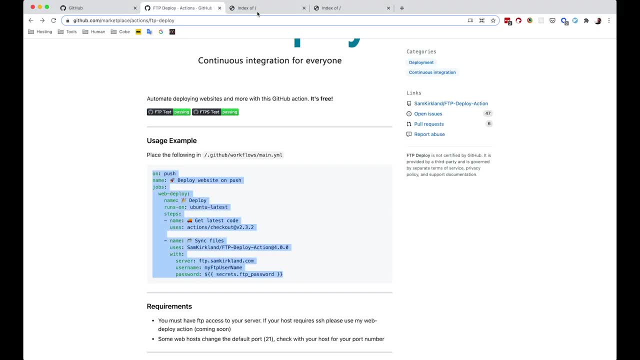 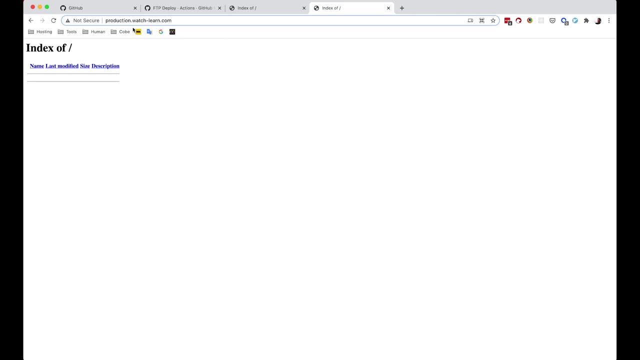 And let me just show you how that looks. So if we go to our browser, I have stagingwatchlearncom- If I refresh it, as you can see, it has nothing in it as of yet- And also I have productionwatchlearncom, which is also just an mp3. 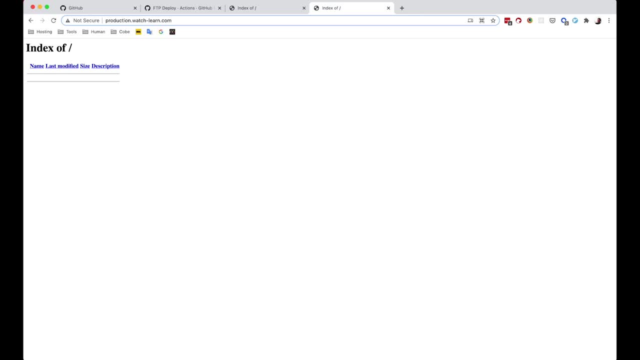 And also I have productionwatchlearncom, which is also just an mp3.. And also I have productionwatchlearncom, which is also just an mp3.. Okay, so, now that we have this set up, let's push our code for the first time to github. 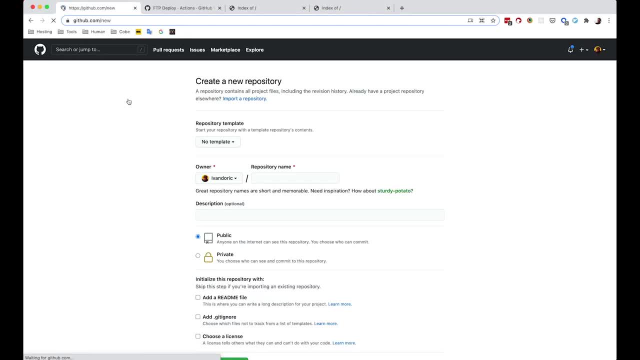 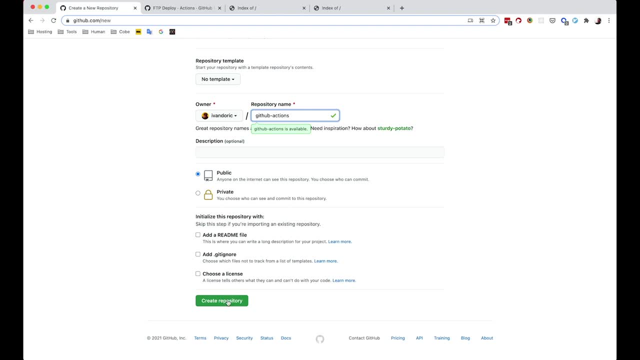 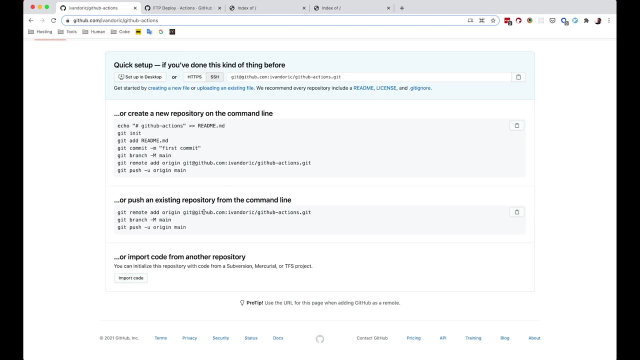 Now I'm just going to create a new repository, I'm going to call it github actions and it's just going to be public directory and that's about it. So we create the repository and now you can follow these instructions right here. We want to push the existing. 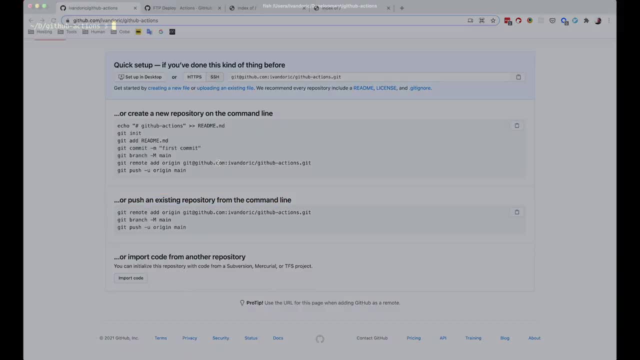 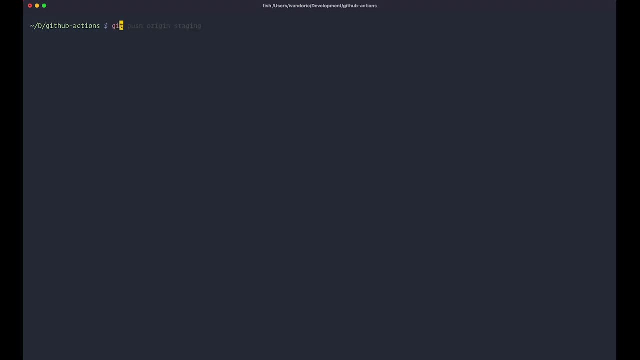 repository from the command line. So first of all I'm just going to go to my directory in my terminal and I'm just going to do git init so that we initialize our git, and then I'm just going to git add something and going to do git commit. it's just going to be first commit, first commit. 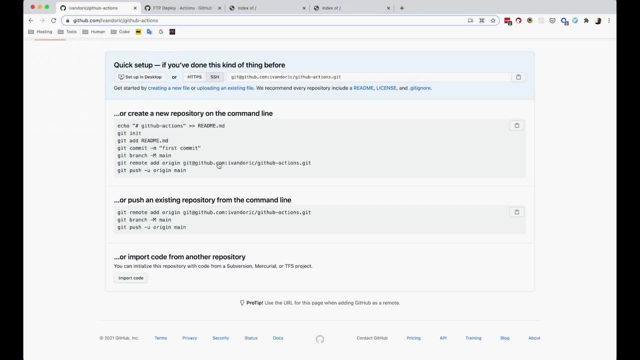 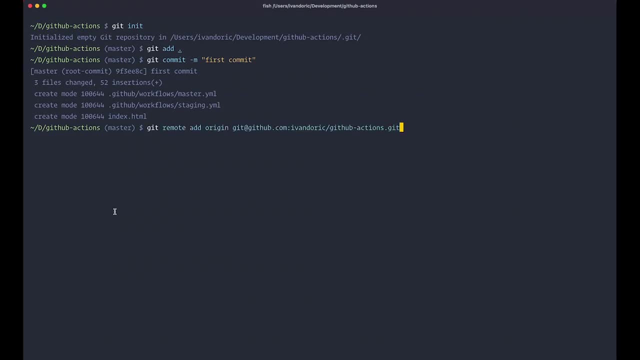 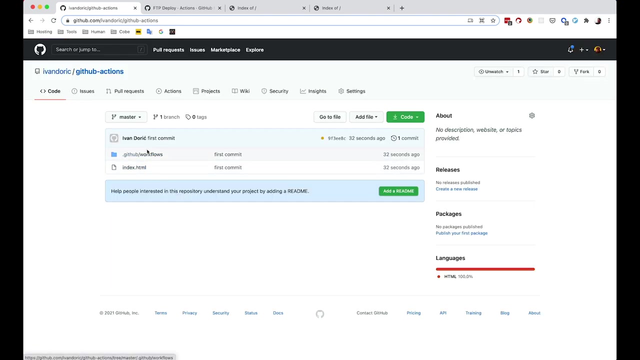 and now I'm going to go to the github and add that This. so we are just going to add git add origin, so that git knows where to push our files, and now all we have to do is do git push origin master. Okay, great, now, if we go to github, refresh this page. as you can see, now we have some files and 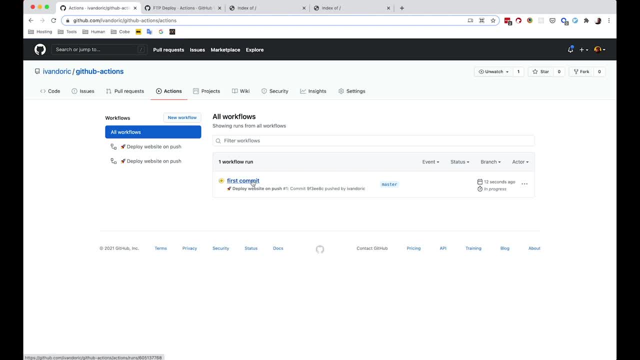 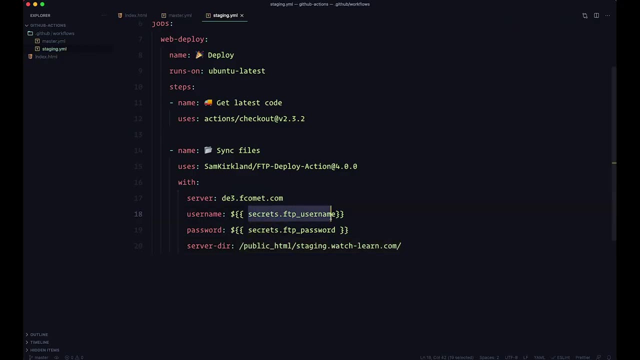 folders in it and if you go to actions, You already see, you can already see that our first commit is actually committing and the github actions are doing something. Of course, this is going to fail. and this is going to fail because we defined these secrets right here. So ftp username and ftp password, but git. 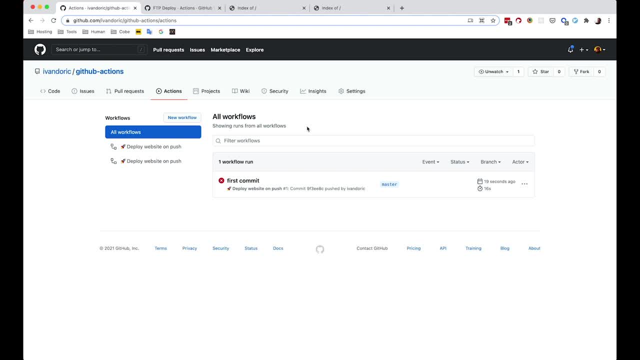 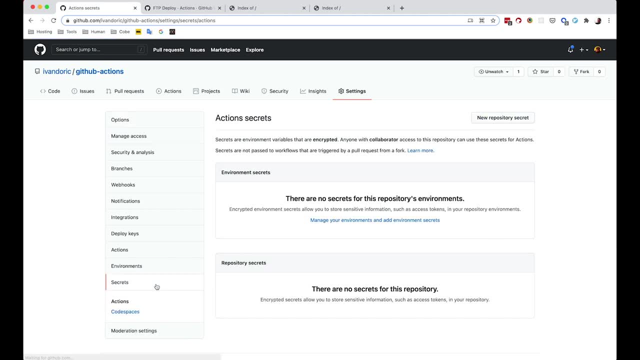 does not have those secrets set up just yet. So how do you set up those secrets? So you go to settings for your project, you go to secrets, And now, here you create new repository secret. Click it and, as you can see, it's called action. 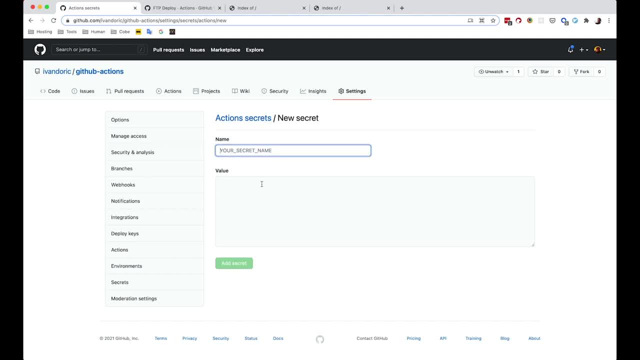 secrets, new secret. So the first secret is going to be called ftp username, and here you would add your username for your ftp, of course, and you can just add a secret. Now you can add a new repository secret, which is going to be called ftp password, just like we defined. 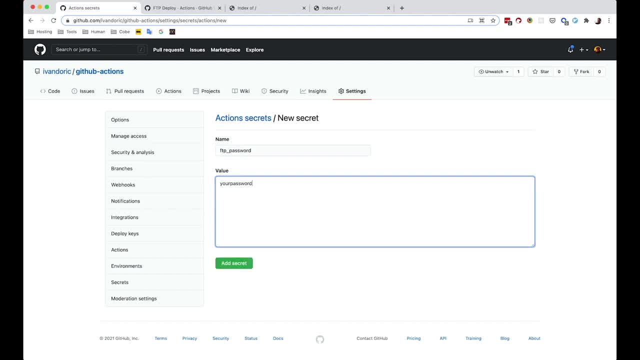 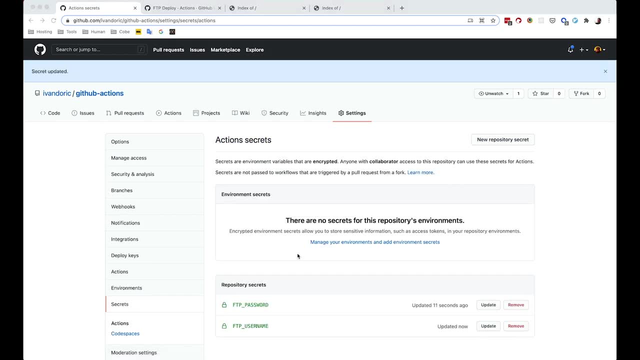 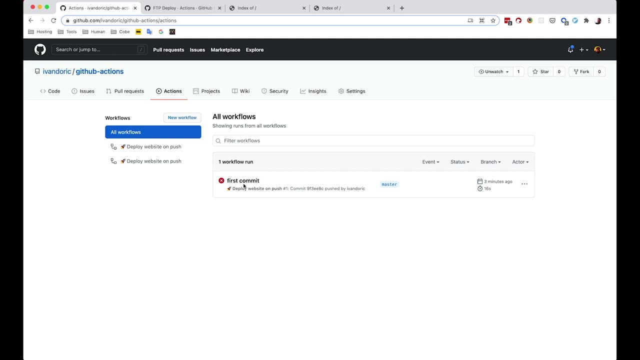 And your password, of course, your password for your ftp and you just add that secret. Now that you have added your username and your password secrets, you can go to actions again. You can click on this first commit and you can click right here: rerun jobs. 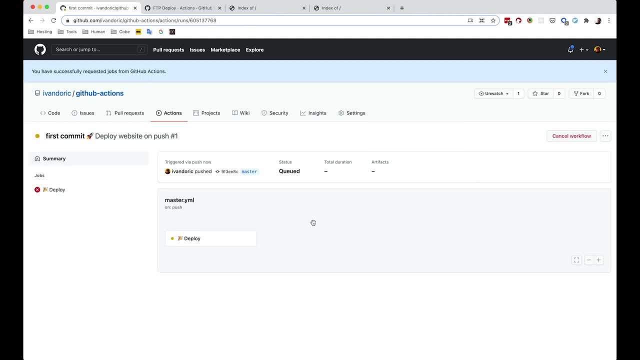 And you say: rerun all jobs and then you wait a little bit for this deploy to be finished And, as you can see right now it says our deployment is finished and you can click right here to see all of the details. So setting up the job. 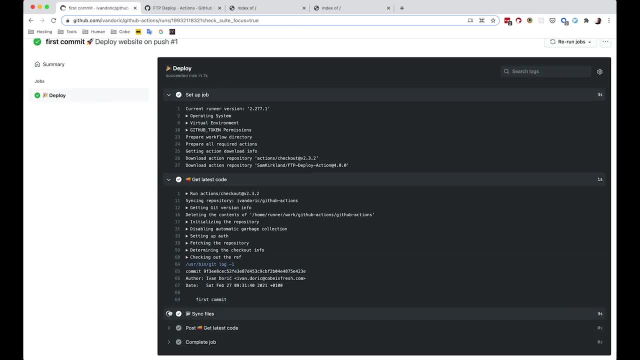 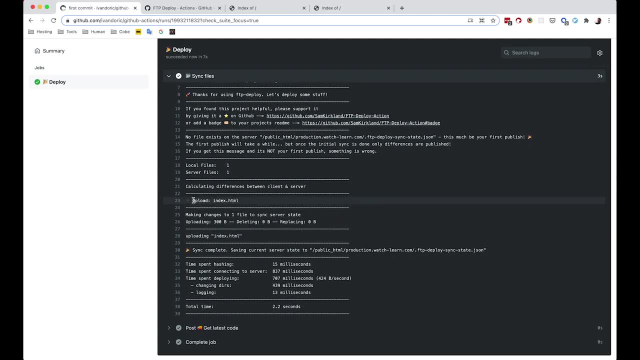 getting the latest code syncing the files and so on, So you can check out what is actually going on right here. So, as you can see, we are uploading the index HTML to our public HTML production watch, learn and so on. So, if I now go to my production server, 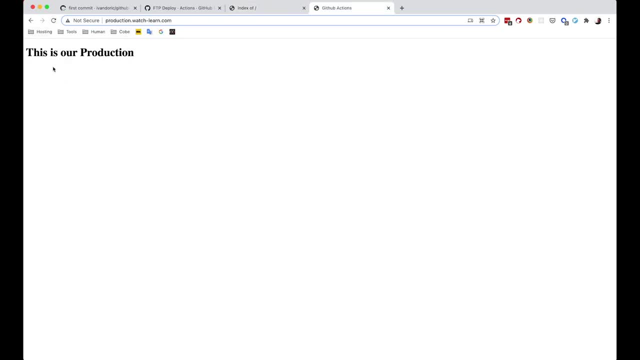 productionwatchlearncom save it. as you can see, this is our production. okay, great. so now let's push something to our staging server, and first of all, we are just going to create a branch, we are going to merge that branch to the staging branch and then we are going to push all of that. 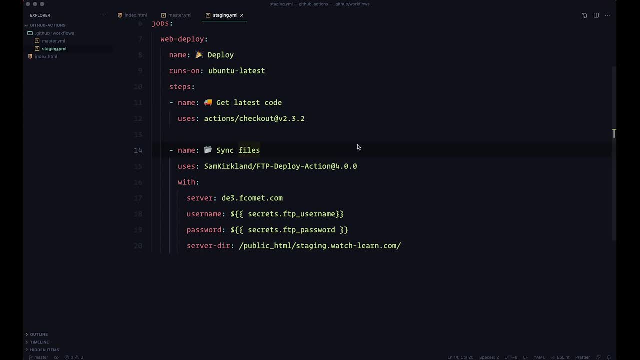 to github. so, first of all, i'm going to create a new branch, so git create branch and i'm going to call it staging. okay, and now i'm on a staging branch, now i'm going to return to master, check out to master and now, from here, i'm going to create another branch which is going to 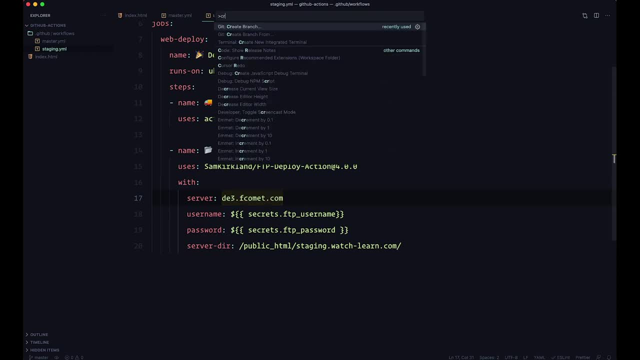 be called new feature. you should always create your feature branches from master because if you have some other things going on on your staging branch, you should always create your feature branches from master branch. that could conflict what you're doing with things on the master branch, of course. 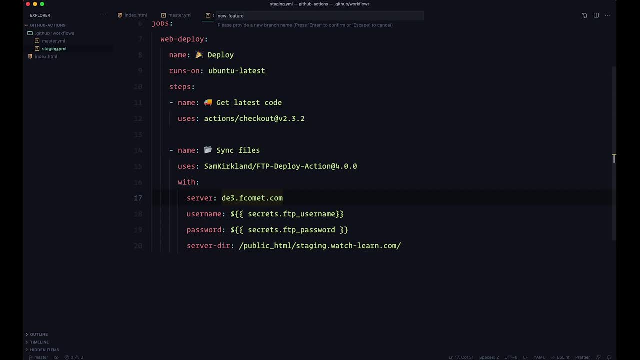 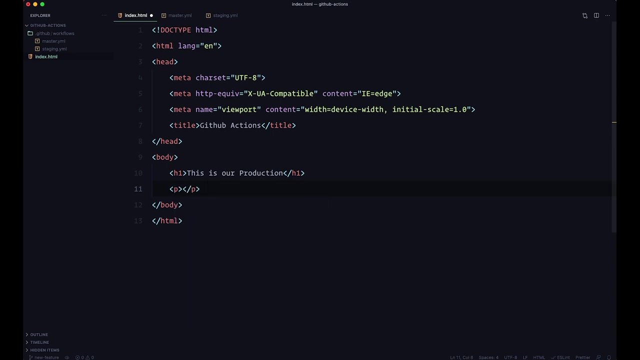 so your master branch should always be clean and have all the approved features in it. so i'm just going to call this new feature. okay, so now we are on the feature branch and now i'm just going to go into indexhtml and do so. p. this is our new feature. 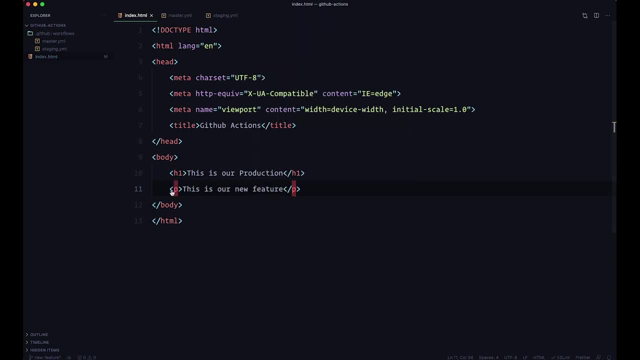 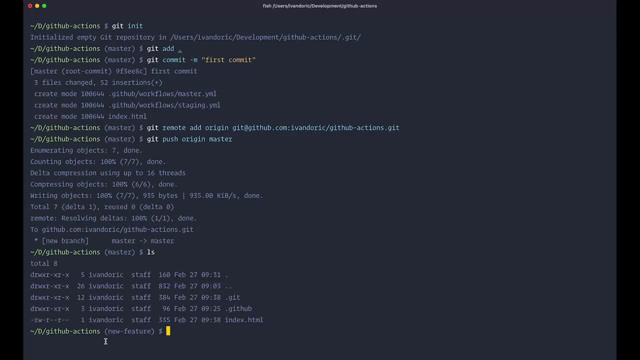 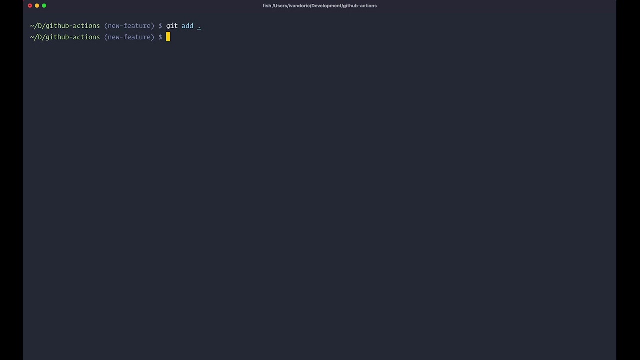 okay, save this. and now i'm just going to go to my terminal and here, if i do ls, as you can see, i'm currently in a feature branch. in new feature branch i'm going to go and git add everything, git commit new feature and i'm going to push this to the new. 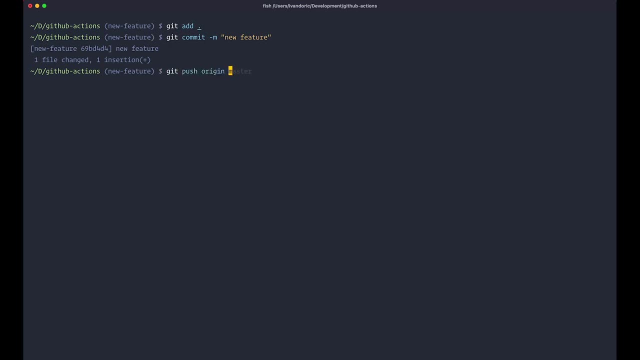 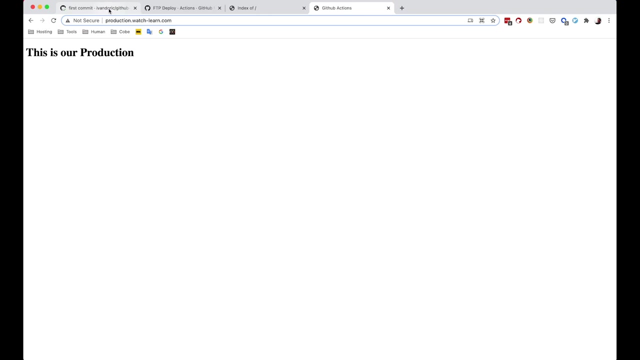 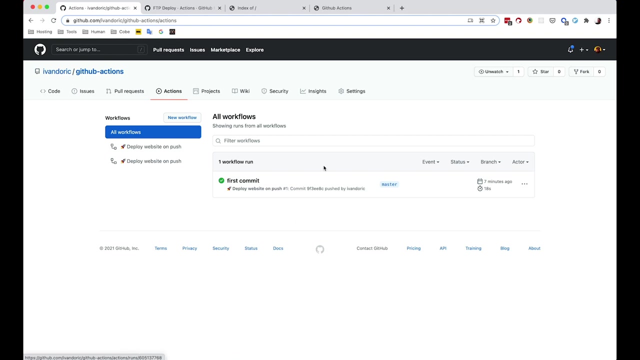 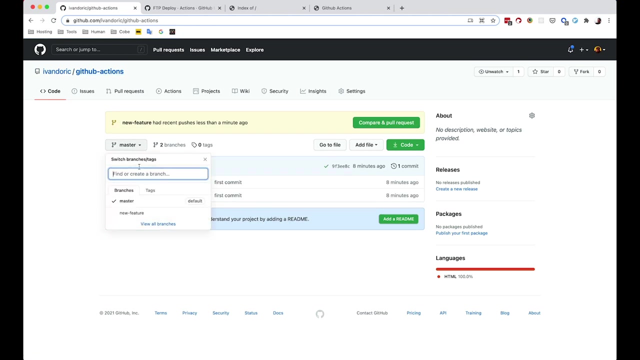 feature branch: git push origin new feature. okay, so git push origin new feature. we push this to the feature branch. and now, if we go to our github repository, so right here and we go to actions, as you can see nothing is happening right now. but we pushed something to the feature branch and, as you can see, we have. 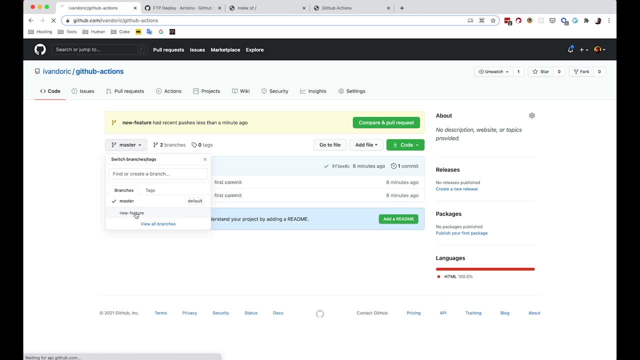 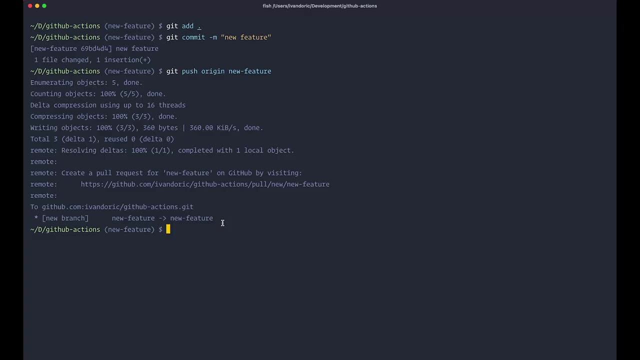 master branch and the new feature branch right here. right, so nothing is happening because we, of course, we defined github actions to trigger only when you push something to master and only when you push something to staging. okay, so now in our terminal i'm just going to check out to the staging branch. 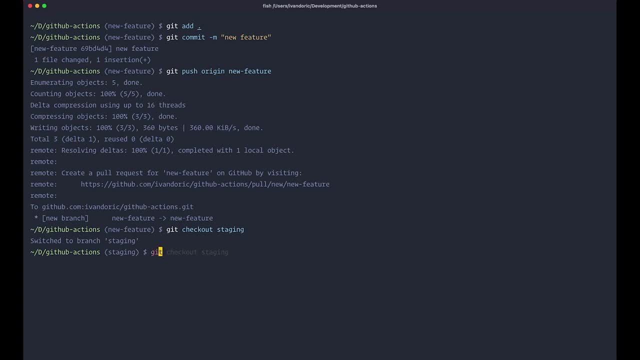 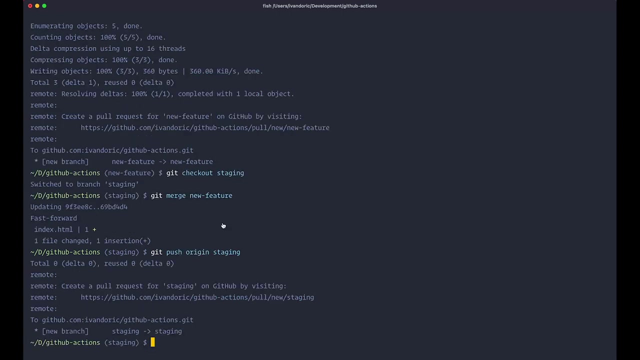 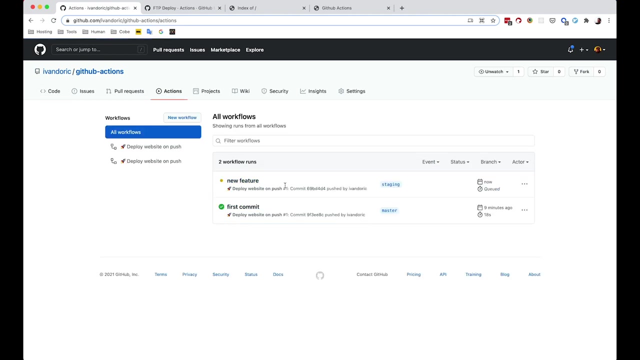 and i'm going to merge new feature branch into the staging branch. new feature: i'm going to git push origin staging and now we are pushing something to the staging branch. now, if we go to our github actions, as you can see, now this is deploying. we are going to just wait just a little bit for this to be deployed. 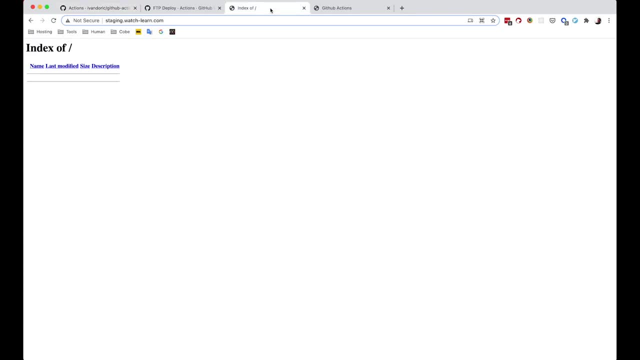 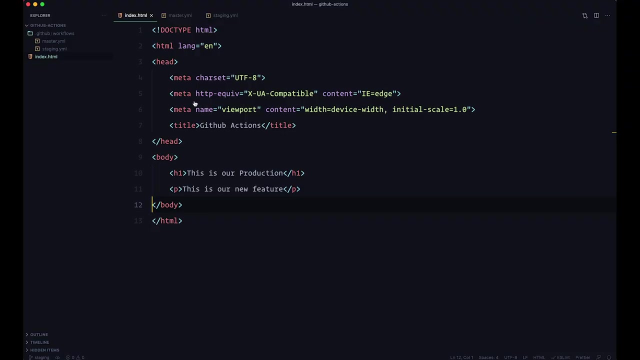 okay, so now that this has deployed, we can check out our stagingwatchlearncom and, as you can see, it says it still says this is our production branch, because because i didn't change that, but it has this. this is our new feature, so i can go to staging again and change this. this is our staging. 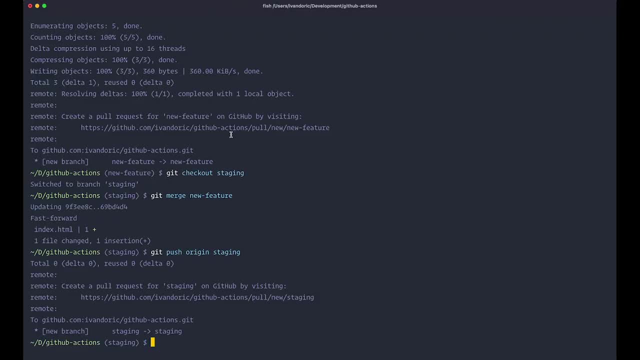 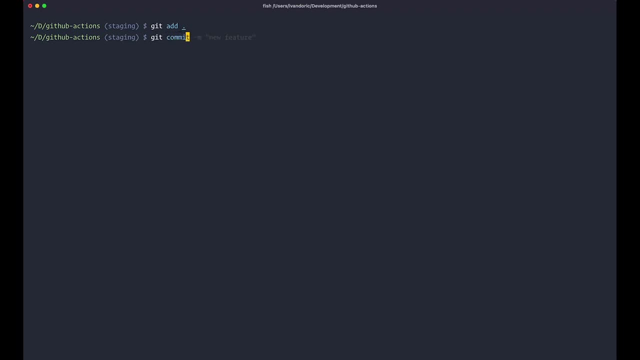 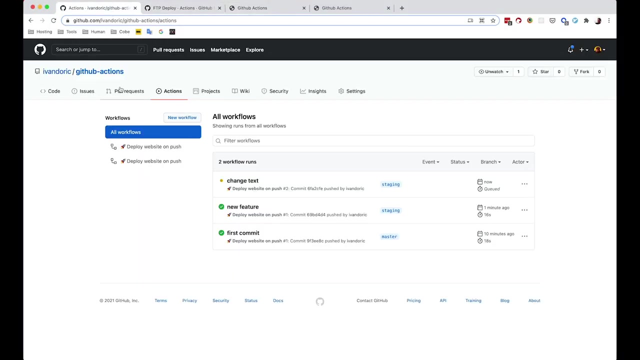 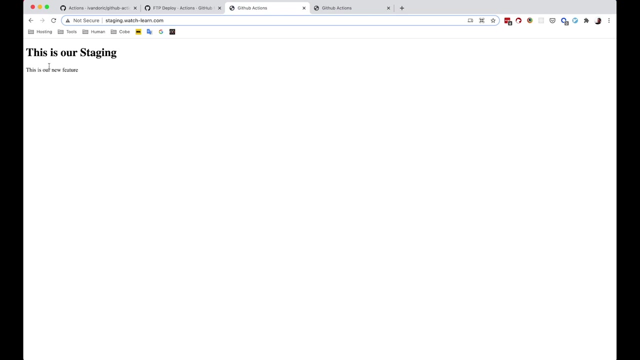 just to be more clear. and we go to our terminal and just do git, add, git commit and just push it to staging. go to our browser, check if this works. as you can see, change text is currently deploying. so now, if we go right here, it says this is our staging.